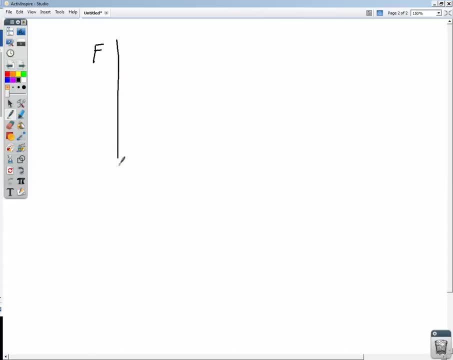 Again, we're going to graph force on the vertical axis and we're going to graph displacement or position on the horizontal axis. And let's say that for the first amount of time we're doing a force f1, and then we get tired and the force that we apply is less. 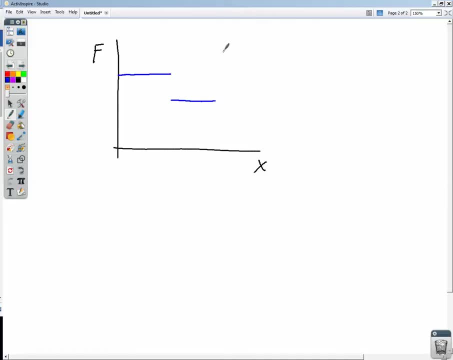 That would be f2, maybe, And then we get told by our boss to hurry up, and so we apply a greater force this time. So we've got f1,, f2, and f3.. So this is a changing force and it doesn't change instantaneously. 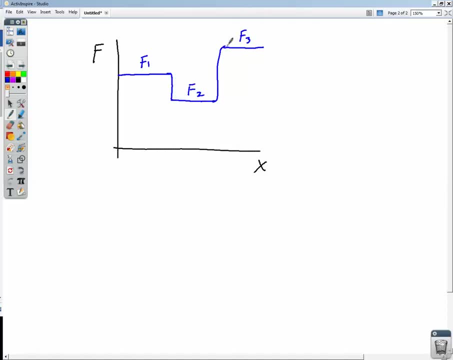 but it changes pretty quickly. So we want to know the total work done in this entire displacement in moving this object from some position 0 all the way out here to position x, And again, as we saw, it's just the area under the curve. 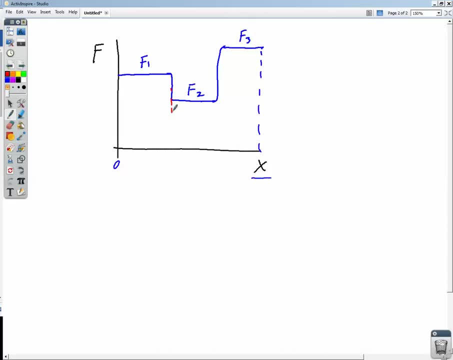 So this is really easy to find the area between these curves, because we have three rectangles And we would do f1 times this first displacement, x1 minus 0. And then we go here and do f2 times this displacement, which is x2 minus x1. 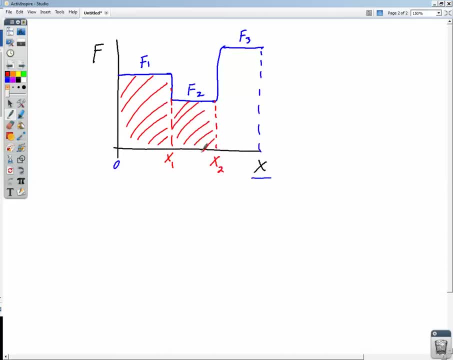 That'll give us the area of that rectangle. And then finally, we would do f3 times this displacement here- x minus x2, and that gives us the area of that rectangle. So we get this And again, the area under the curve is going to be the work done. 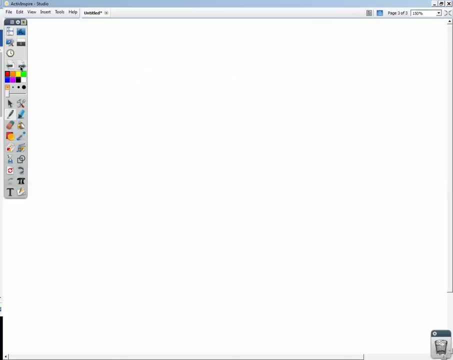 All right. So let's take a look at what this looks like for a spring, an ideal spring. So this is a work done by an ideal spring, And remember that when we say ideal spring, we're talking about a spring that conforms to Hooke's law. 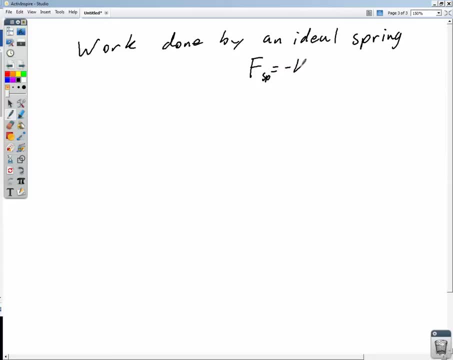 The force applied by the spring is equal to negative kx. The force and the displacement are in opposite directions. Let's take a look at a specific situation here. Let's say we've got a spring attached to a wall and we've compressed the spring. 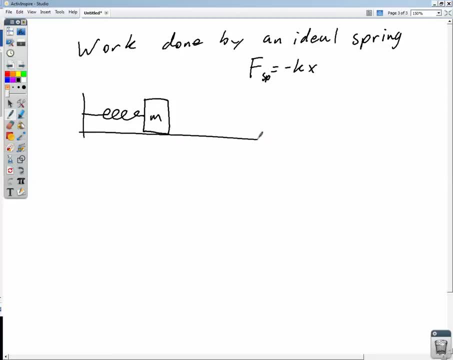 and we've put a mass m on the end of this spring. It's sitting on a frictionless surface and we have compressed the spring by some delta x here from its rest position And we're going to let this mass go, And we know that as we let the mass go, 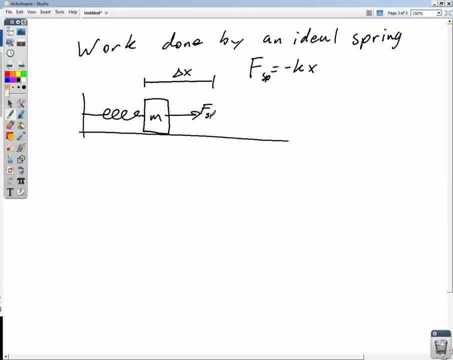 the spring is going to apply a force on the mass to the right And as that mass moves to the right, accelerates to the right, the force applied by the spring gets less and less and less because that delta x gets smaller and smaller and smaller. 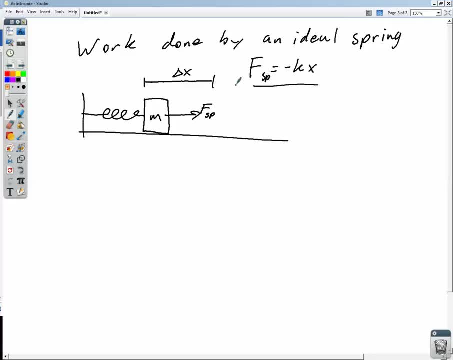 And we know that the force applied by the spring is equal to that negative kx. So if we graphed this- the force versus the position of the spring- the force starts out at its maximum because it's displaced its largest amount, And then, as the displaced mass, 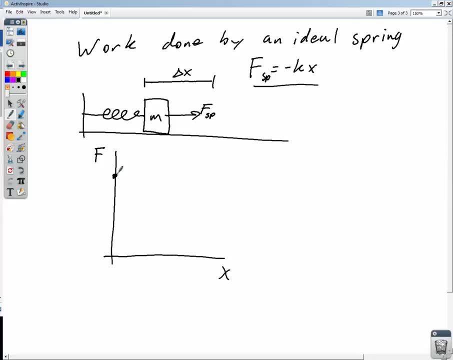 gets smaller and smaller and smaller. wait, let me think about that for a second Correction. the force doesn't start out here, The force starts out here at its maximum. So for the biggest displacement, delta x, you're going to get the biggest amount of force. 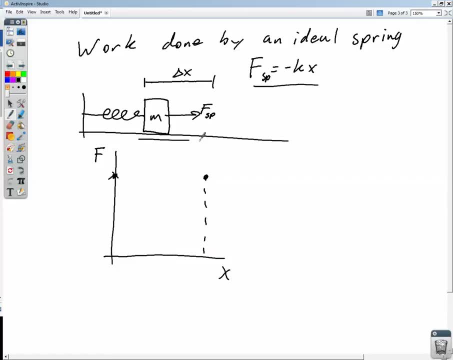 So that is this situation. right up here, The block is at rest. We're ready to let it go Now as the displacement gets smaller and smaller and smaller as the spring moves back towards its rest position. eventually, when spring gets at its rest position, 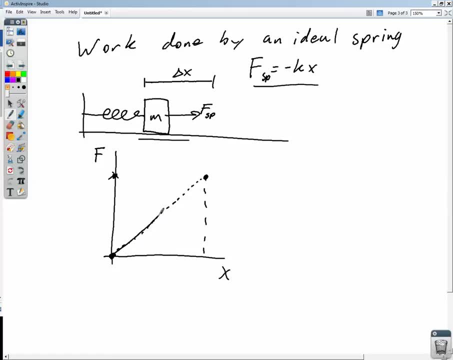 the force is going to be zero, and so is x the displacement. So now we've got this situation right here And that should look familiar from class the other day when we did our lab stretching the spring. We get a nice little linear force versus position graph. 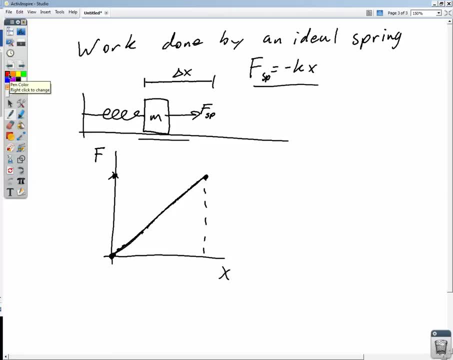 Now, what we found before was that the area under the force versus position graph is going to give us the work done. So if I want the work done by the spring, I'm looking at the area of that triangle Now, so the bottom of the triangle, the base of the triangle. 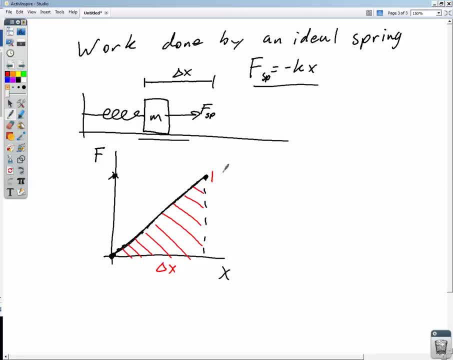 is our delta x And the very top of the triangle. the height is this: f. at whatever that position, x was the maximum displacement. So if I want to know the work done, it's going to be the area of this triangle. 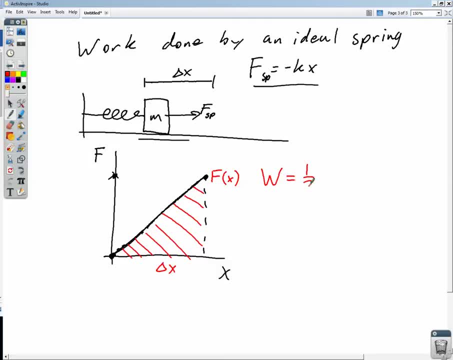 So area of a triangle is half the base times the height. So half the base is half of delta x times the height here, which is the force, that maximum force at the position x. But we know from Hooke's Law that f is equal to kx. 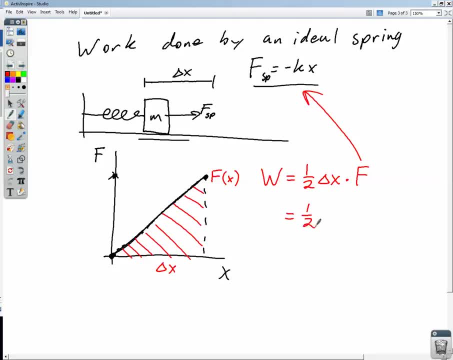 So the work done here is going to be half of. let's just, instead of saying delta x, we'll just say x half of x times that f, which is kx. All right, The force on the spring is positive here. 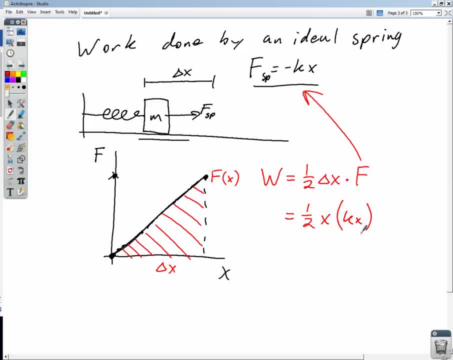 so I'm going to make my kx positive, And so then we get the work done by the spring: 1 half kx squared, And this is a general equation that holds for any ideal spring, any spring that conforms to Hooke's Law. 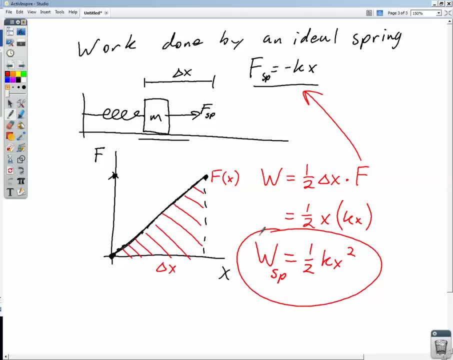 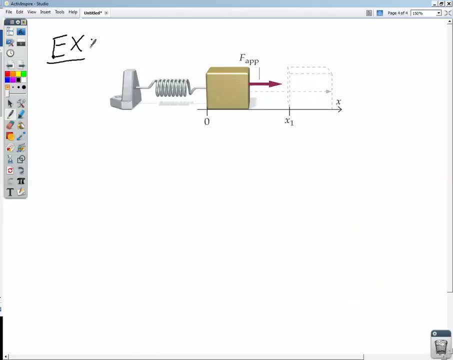 The work done by the spring is 1 half kx squared. Very worth remembering, and I'm pretty darn sure it's on your equation sheet as well. But we can double check that, Okay. so let's look at an example here. 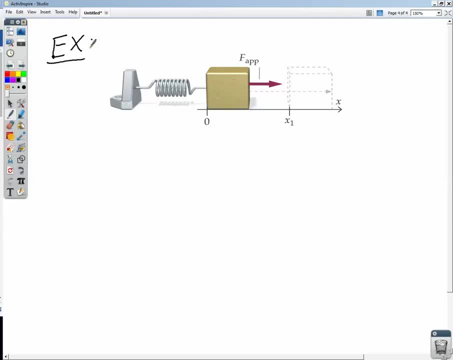 And it's the same example we just looked at. We've got a spring that's compressed and it is going to accelerate this block all the way to this position x1. And then the block's going to get released and it's going to cruise. 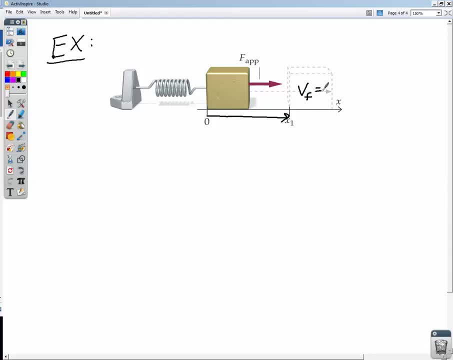 And we want to know what is the velocity of the block right here when the spring is done, pushing it All right. So we can use the work energy theorem to answer this question, because we remember that the net work done on an object is equal to the change in kinetic energy. 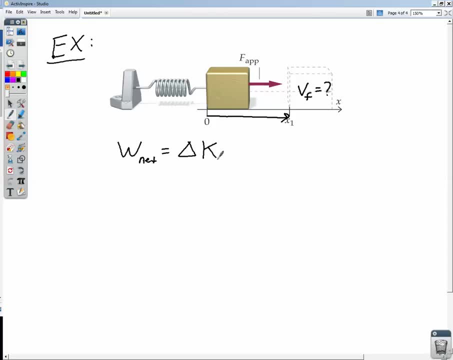 And this is going to allow us to relate the force that the spring applies over the distance to the change in the kinetic energy, which is going to allow us to relate it to velocity. We could not have answered this question using Newton's laws and kinematic equations. 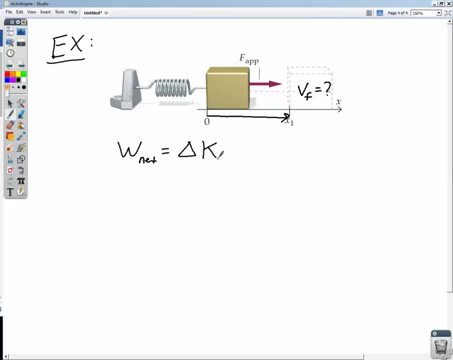 because the acceleration of the block while the spring is pushing it is not constant. Quick free body diagram for the block. We've got this applied force, which is the spring force. We've also got mg going down. We've got the normal force going up. 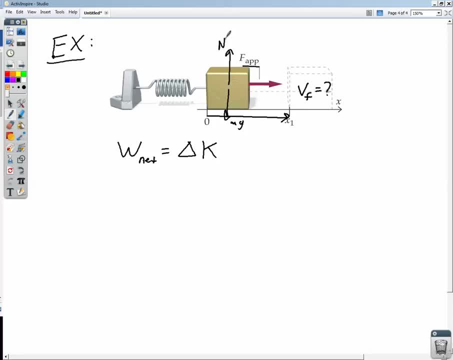 There is no friction between the block and the surface. So it's easy to see here that the weight doesn't do any work because it's at a right angle to the displacement. The normal force doesn't do any work because it's at a right angle to the displacement. 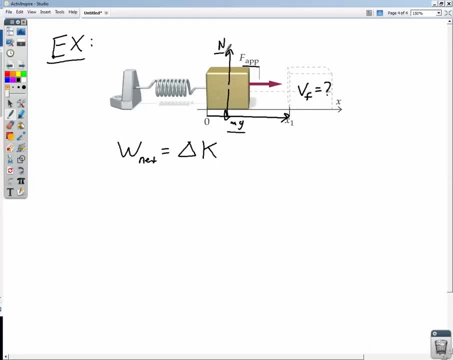 So the only thing that does work is the spring force. So we can say that the work done by the spring in this case is going to equal the change in the kinetic energy: k final minus k initial. And let's see here k initial: it starts at rest. 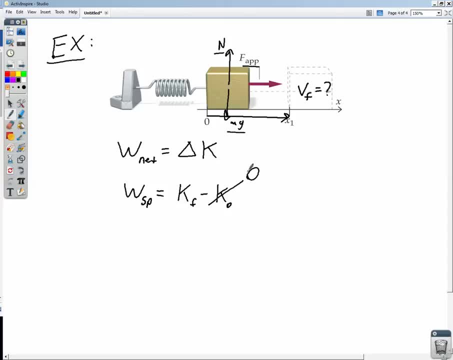 So this guy right here is zero. That simplifies our equation dramatically. So the work done by the spring- we already learned in the previous one- is 1 half k x squared. And I'm going to say: be careful with the work done by the spring. 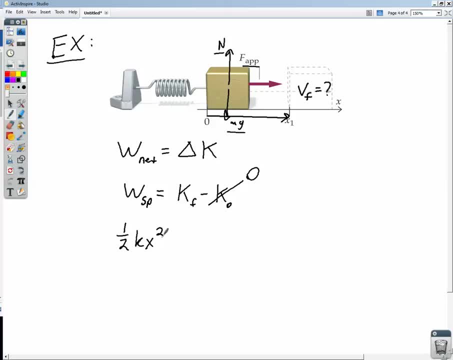 It can be positive or it can be negative. You have to think about the situation and judiciously put in a plus or a minus here in front of the work done by the spring. Just look at the situation. Is the spring's force speeding the object up? 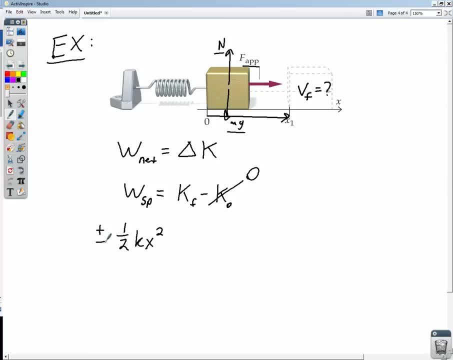 Great The work is positive. Is the spring's force slowing the object down? Great The work is negative. We could easily imagine a reverse situation, where we've got a block out here and it's coming at the spring with a certain velocity. 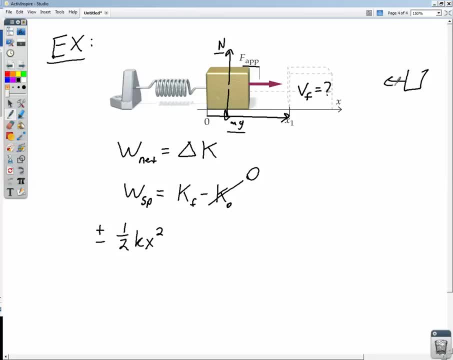 It hits the spring and compresses the spring. In that case the spring is acting to slow it down. We get a negative. We cannot just look at the x, the delta x, to give us positive or negative, because it's squared in the equation. 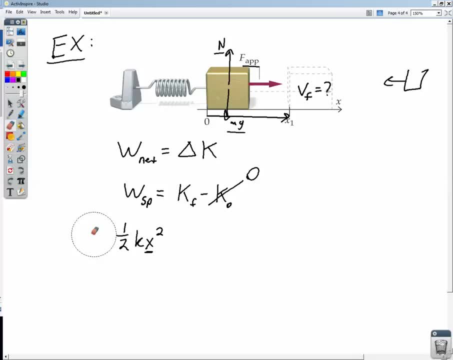 So we have to judiciously determine if the work done by the spring is positive or negative. In this case it is positive because it's speeding up the block, And this is going to equal 1 half m v final squared. Notice: mass does not cancel out. 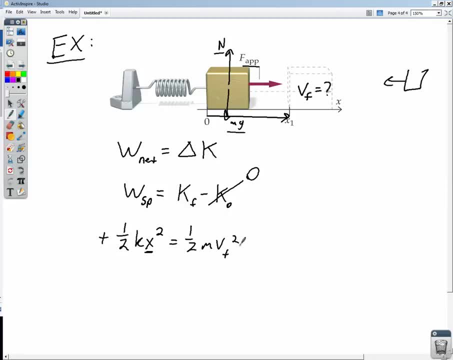 when we're dealing with spring problems, because I don't have an m on the left-hand side, We are looking for v, final squared. The halves do cancel. Dividing by m and taking the square root, we have k, x squared over m. 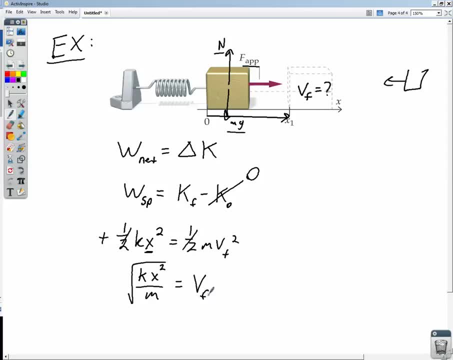 We take the square root of that, That is equal to v final. If you wanted to clean it up a little bit, you could say x times the square root of k over m, because that x squared comes out from under the radical, And that's equal to v final. 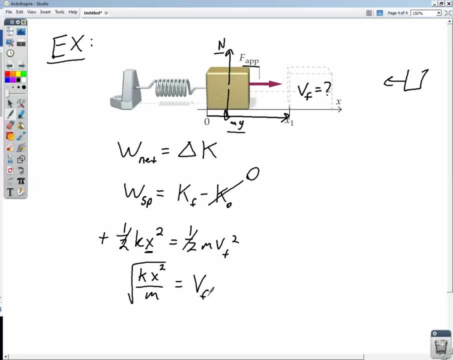 But that's the basic situation right there. So with this setup, keep in mind that we could solve for k. if we had the opposite situation, where the velocity was coming in, The block was coming in and hitting the spring and compressing it, We could solve for k.